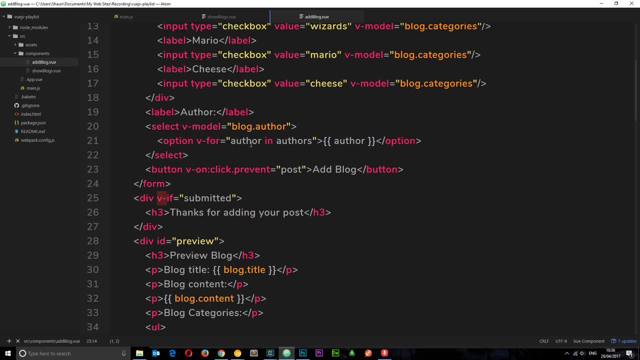 So what if we want to do something in Vuejs, we want to use a directive, But that directive doesn't exist. the behavior we want Isn't already included in Vuejs. Well, we can create a custom directive, which is what I'm going to show you how to do in this tutorial. 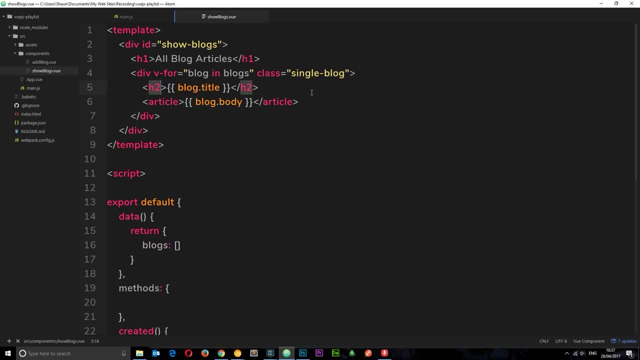 So I'm going to go to our show blogs Component right here and say, for example, this blog title we output, but I'll put in ten of them right on the page. Say, I want each one to be some kind of random color, right, So we could make up our own directive and 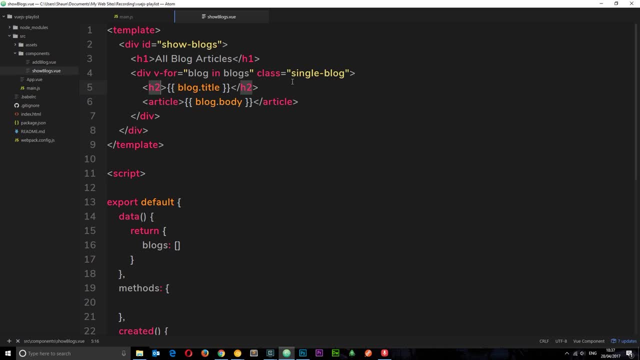 We could control that functionality. So if I want to add a directive, I could just say V, hyphen. then, whatever the directive Name is going to be called, now We'll make one called rainbow which is going to do this. So it's just going to choose a random color and assign it to each h2.. All right, 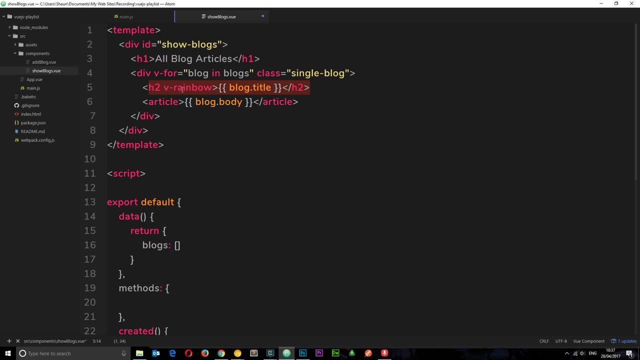 So each h2 on the page is going to be a different color. So we've got this directive right here. We don't need to set it equal to anything. I mean, we can do, and we'll do that later on, but we don't have to do that. 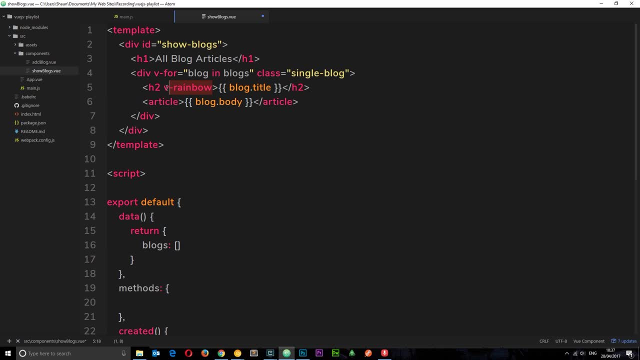 We could just have a bog, standard, simple directive- V- rainbow- Which, when we apply that to an element, is going to give it a random color. Okay, so let's save this and let's create this directive. So we're going to create this globally, this directive, and I'm going to show you how to do things locally later on, in later tutorials. 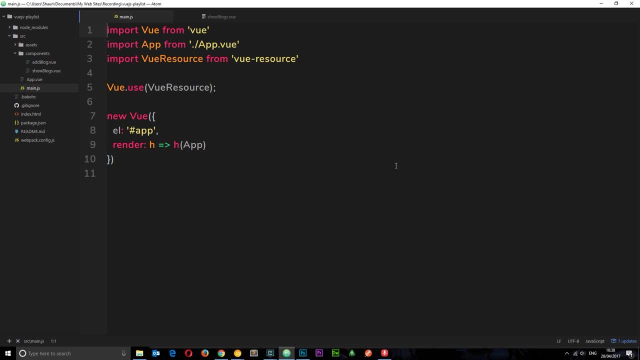 But for now, let's just create a directive which is going to be global, meaning any component can use it. So the way we're going to do this, first of all, is go to mainjs and then let's do a little comment saying custom directives. Okay, then, the way we create a directive is by saying it: view. 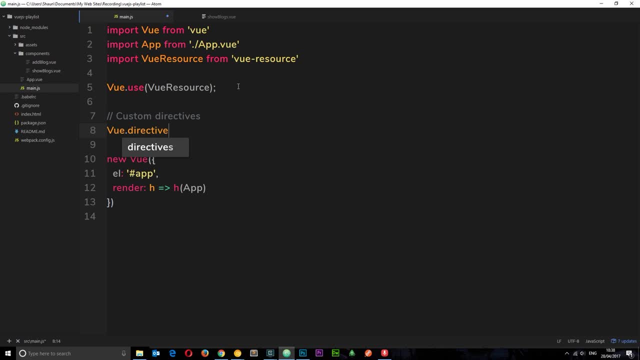 Directive. so this is much like when we created a component, We said view component. this time it's viewed our directive. Okay, and this takes a couple of arguments. first of all, the name of our directive. now, Remember, we call this V hyphen rainbow, but this isn't the whole directive name. This bit is the directive name. 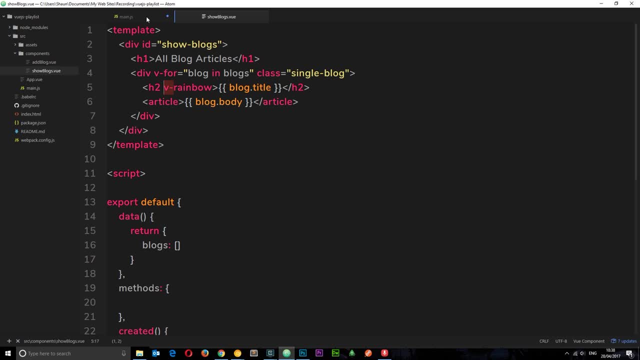 Okay, this is just something we put before the directive name, So in here we want to just call it rainbow. Okay, then the second parameter right here is going to be an object, and inside this object is where we can control the functionality of this directive. 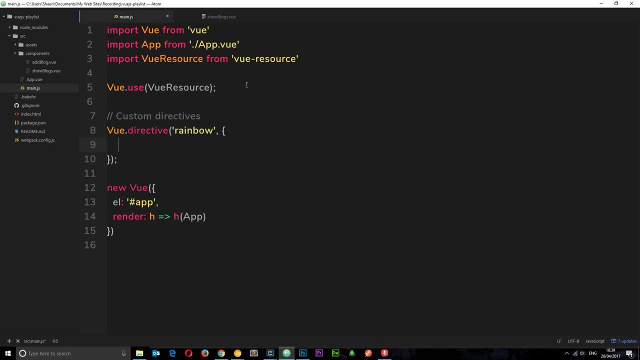 Now you know, like in previous tutorials I said, that components have lifecycle hooks, like created, destroyed, updated, that kind of thing. well, soda directives and We're going to use a lifecycle hook called bind and basically what this does is fire When the directive is bound to the element, so as soon as it kind of hooks up, if you like. 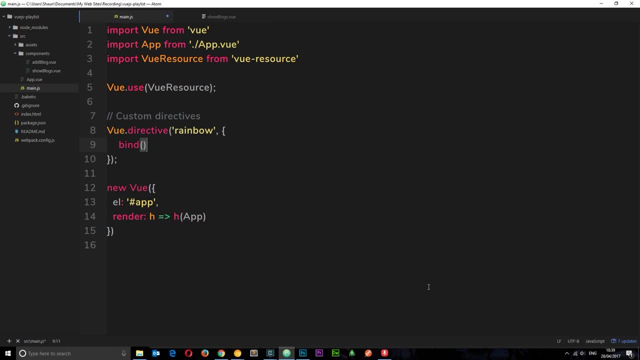 okay. so as soon as it's made that kind of connection, we're going to fire this bind function and Inside this function We're going to control what it does. but this bind function right here takes three parameters: L, binding and Virtual node, which is just V node. Now, this thing right here refers to the virtual node on the Dom. 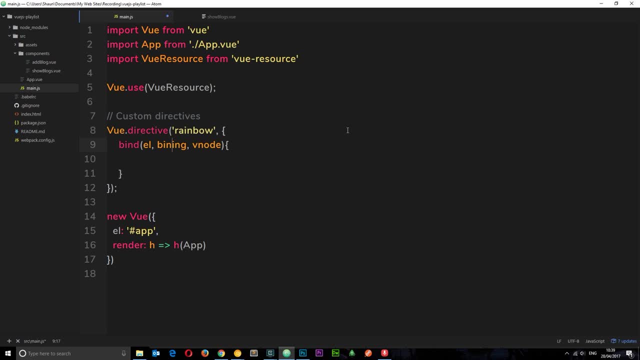 You're not going to need this much. Okay, let's just spell binding correctly. Okay, so we don't really need to touch that this thing right here. binding refers to information about the connection. if we pass it in a value, for example, like this in here: okay, things like that, and we're going to take a look at that shortly, and 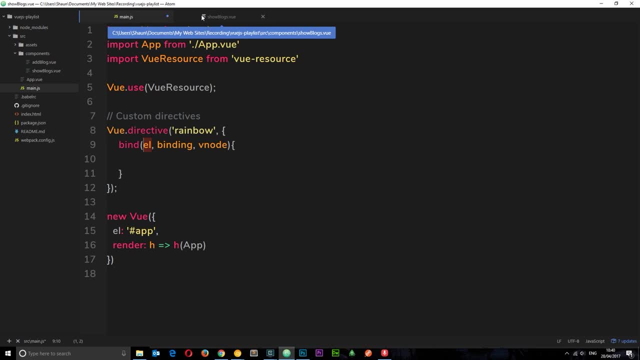 Then this L right here refers to the element itself. So this whole thing that it's on. Okay, So what we can do, for example, for this rainbow component, is take this element and then give it some kind of random background color. Okay, so the way we're going to do that is by getting the L, and then what we can do is just 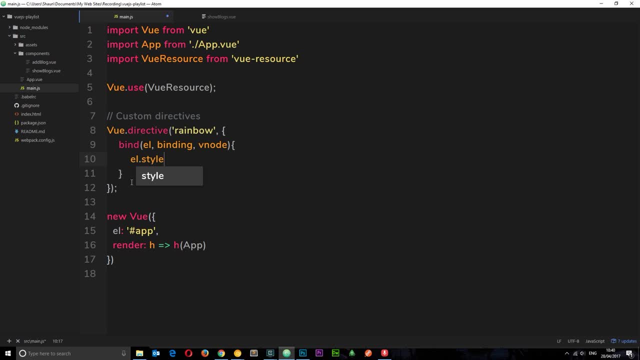 Get the style property of that element. Okay, so this is the CSS Style and then we can decide which property we want to style. we could say: dot color. So that is going to be equal to some random color, right? So what color is it going to be equal to? well, it's going to be a random hash color. 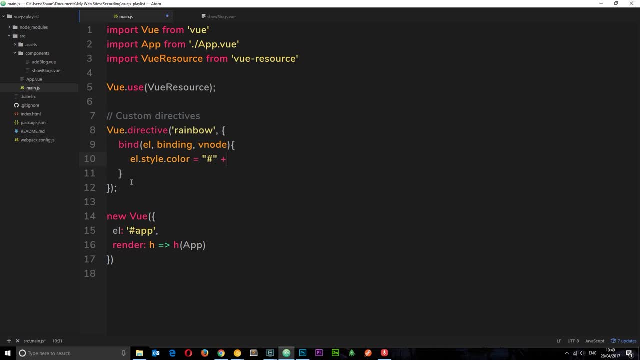 So first of all we need a hash. Then we're going to tack on six random digits. now, how we're going to do this? Well, we're going to use the math object, Okay. then we're going to say: get us a random number. 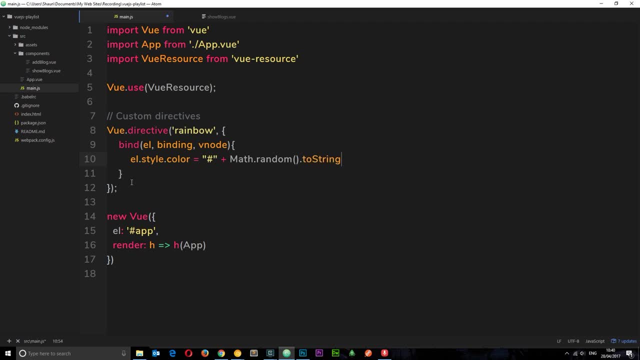 Then we're going to convert that to a string to string and then, finally, What we're going to do is slice that. so we'll say slice Two to eight, and that is going to get us a random six digit number. Okay, so now we could save this. and if we view this in a browser? 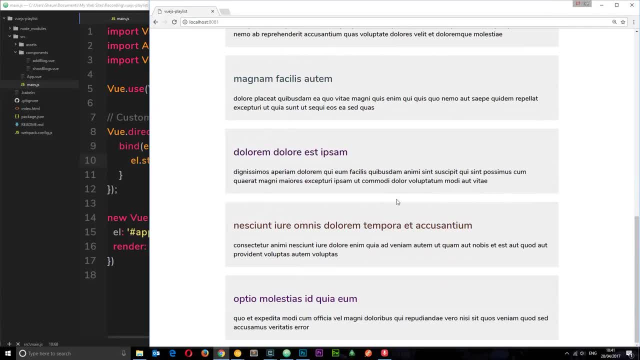 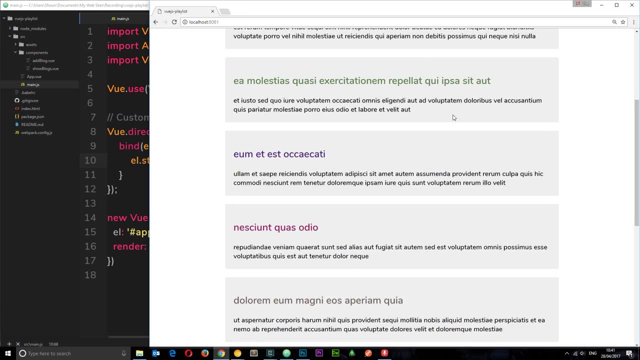 Then we can see that each one of these has a random color. Okay, and if I refresh, then we're gonna get different colors. So they're not hard-coded or anything like that, They're just completely random, which is why I called it V a rainbow. So there we go. 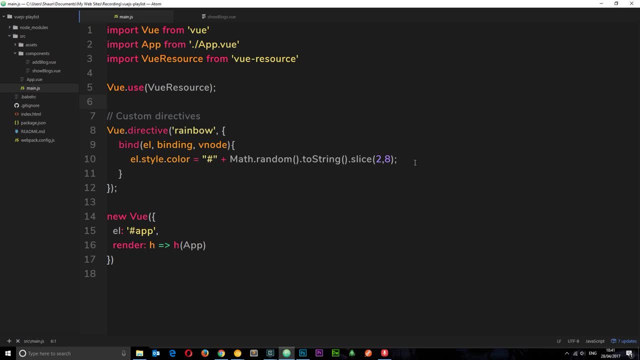 Congratulations: you've made your very own Directive. Okay. Now, if this bit here is confusing, you just do a quick Google search of the math object and random and things like that. This isn't a math JavaScript tutorial, So I'm not going to go into too much depth. 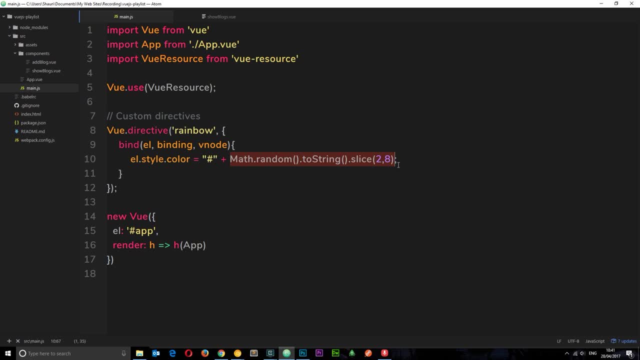 But basically all this is doing is returning to us a six digit random number Which is going to be attached to this pound symbol to make a hex code. But this isn't the point of the tutorial. the point is we can add a directive and we could even do something just like, for example, 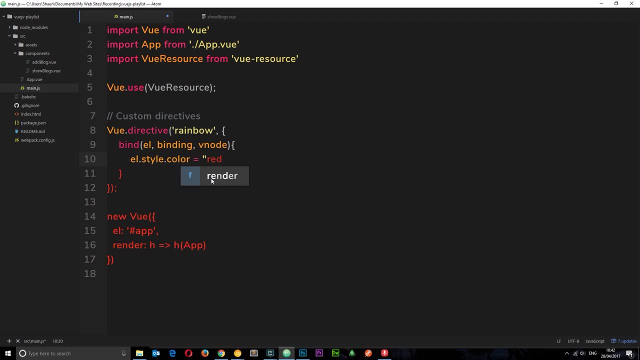 If I copy that out and say read: if we wanted everything to be read, We could do that, save it and everything's read. Okay, I just wanted to make it a random hex code because it's a little bit more fun. Okay, so That is how we make a custom directive. now I said we could do other things. We could do something like this: 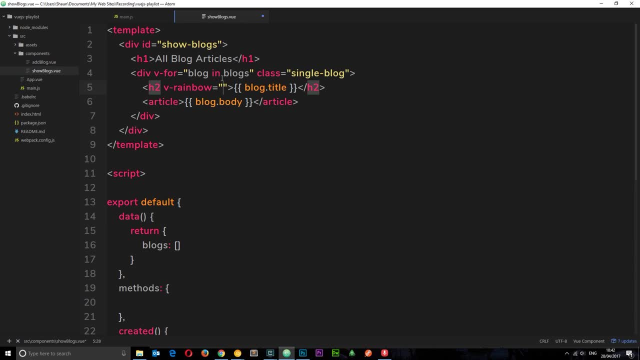 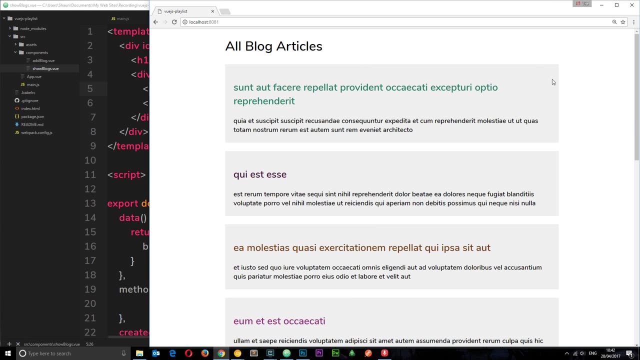 We could say equals and then pass through some kind of value. Okay, so to demonstrate this, I want to create a different custom directive. So this time the directive is gonna Control the kind of like the theme of the web page, and the theme is going to be whether it's going to be a wide 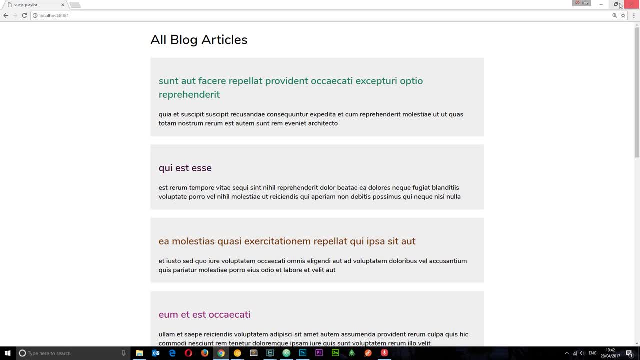 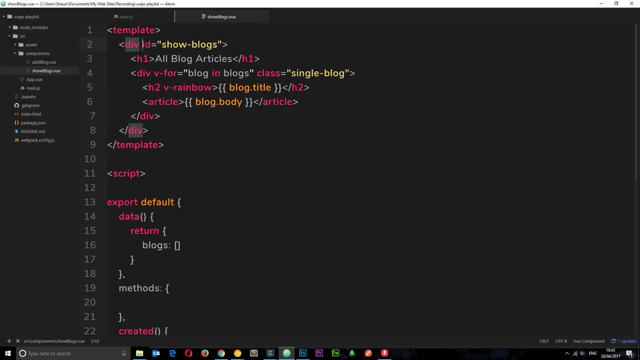 Theme or a narrow theme. Okay, so something pretty simple. So let's attach this directive to this div right here that surrounds all of the blocks, So we'll call this directive theme. So it's V hyphen theme, right? And then we're gonna set that equal to something in a minute. So let's save it for now and 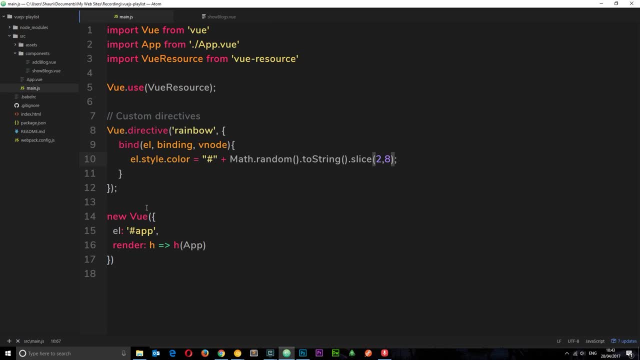 Then inside this mainjs Let's create this directive. So we'll say again: View dot, directive. This is going to register it globally because it's in this mainjs file, So directive. then it's called theme, Then the second parameter is an object and inside this object again We're going to do the bind hook which takes through the L. 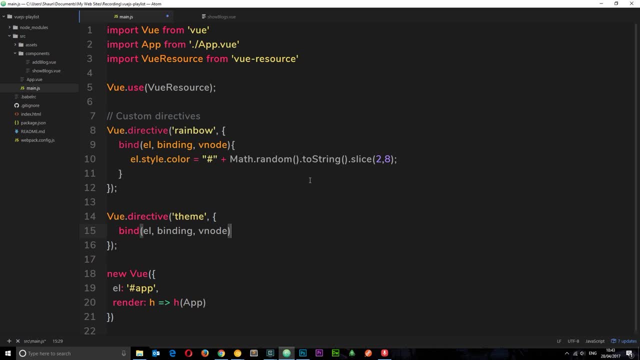 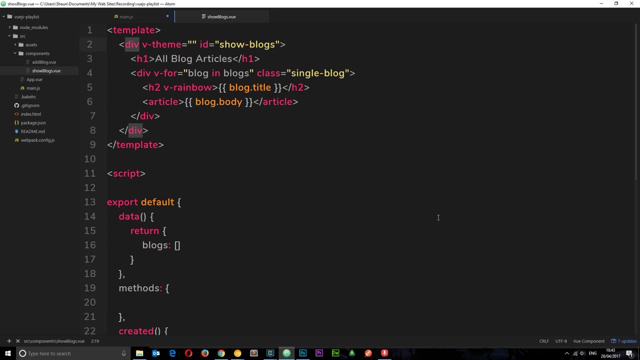 binding and the virtual node. Okay. So now we're gonna give this div right here some kind of theme based on whatever we pass through here. now, Whatever we pass through here, It's going to be called a value, All right. So, for example, if we want a wide theme, we can pass through the value of wide and then we can access. 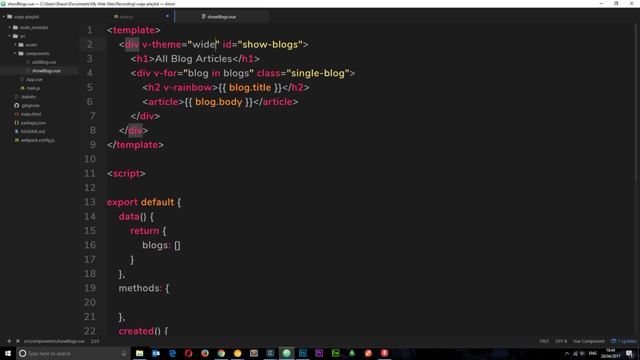 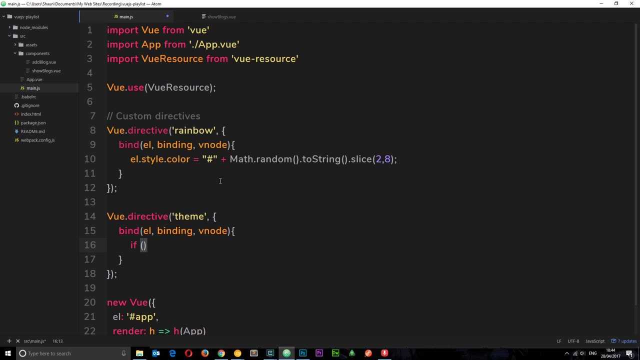 This value right here within the directive we can check to see what value was passed through. So inside here we could say something like if, and then we can say binding, This is going to give us information about the directive and we can get the value property on the binding. 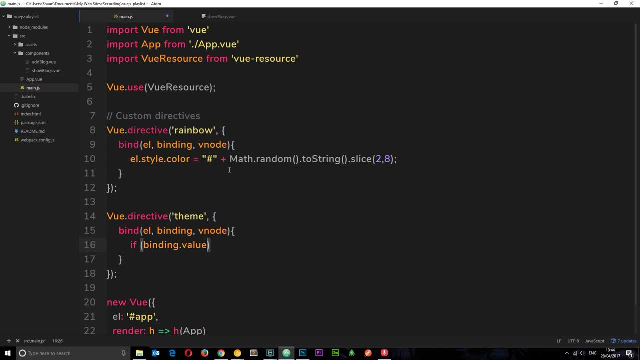 Okay. so we can say, if the binding dot value is equal to Wide, which it is at the minute, Okay, it's equal to wide, That's the value. then we can do something. So what we want to do if it's wide is give it a wide theme. 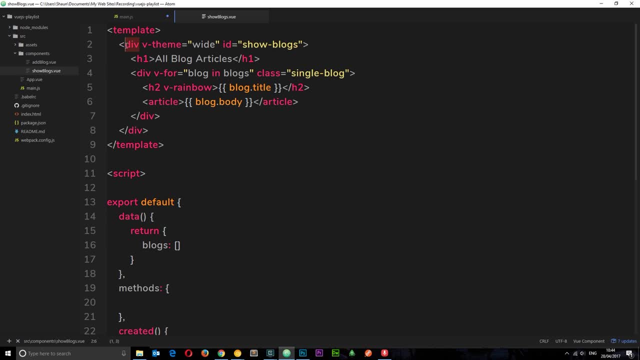 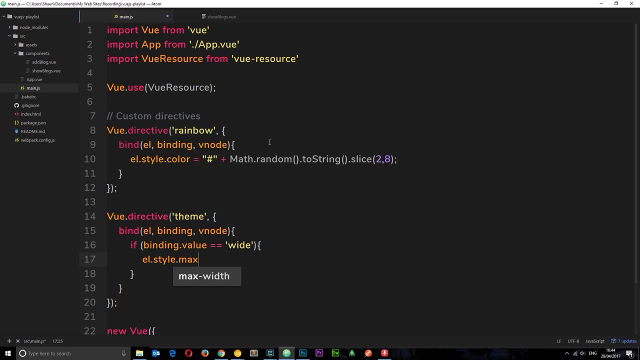 So we'll say L, which is the element. we've attached it to this thing right here, this dig, so we can say L, dot style, dot max-width- And, by the way, when we use two words, it's camel case like that. Okay, We don't say max-height. 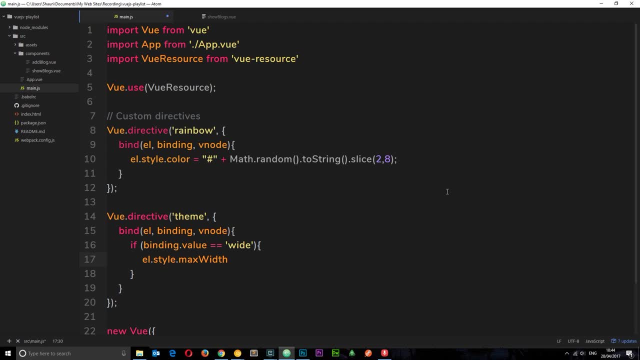 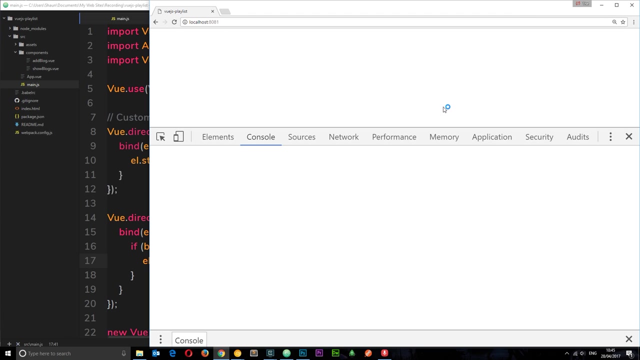 hyphen width or anything like that. it's just max width and we're going to set that equal to 1200 pixels. okay, so that's if it's wide. so if we save this now view in a browser, then refresh. nothing is showing up. so i'm just going to open up the console and see what's gone wrong. 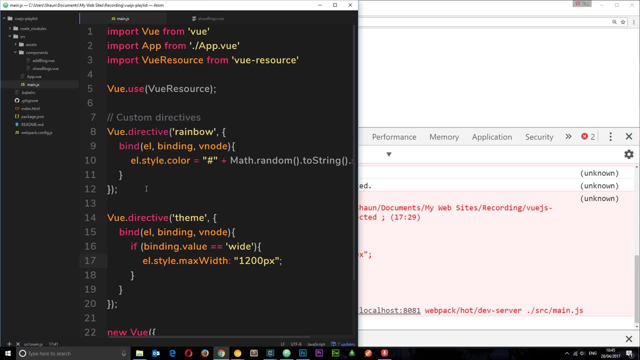 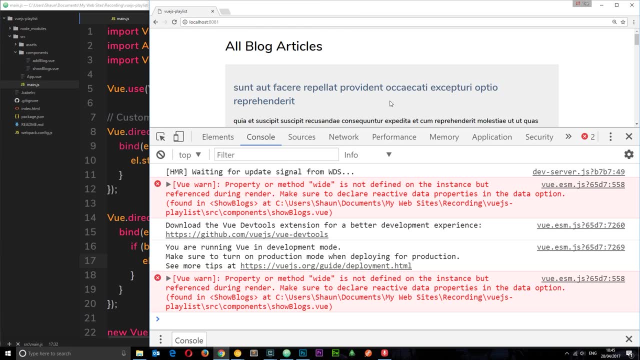 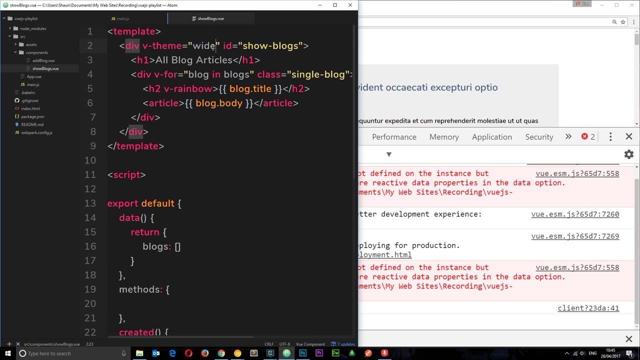 and we have a syntax error. so that's because i've stupidly said colon here instead of equals. so save that and we should get this if we refresh. but we get another error and this is something i actually wanted to show you. so right now i've passed through this right here wide. so why is 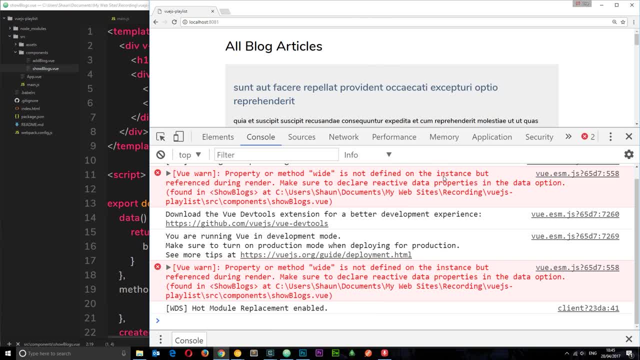 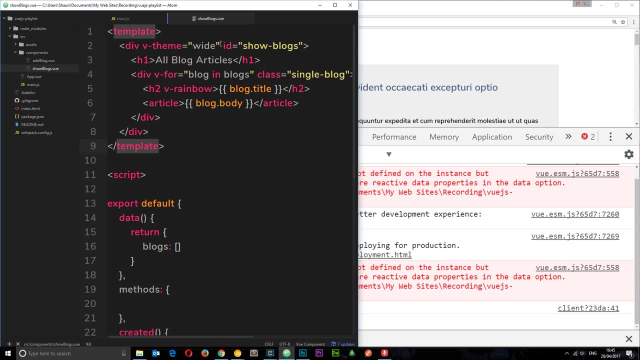 this not working well. it says right here that wide is not defined on the instance, but it's referred during render and it's referred to as a property or method. now, it's not a property or method, it's just a value of passing through here. but because it's a string, we need to pass it. 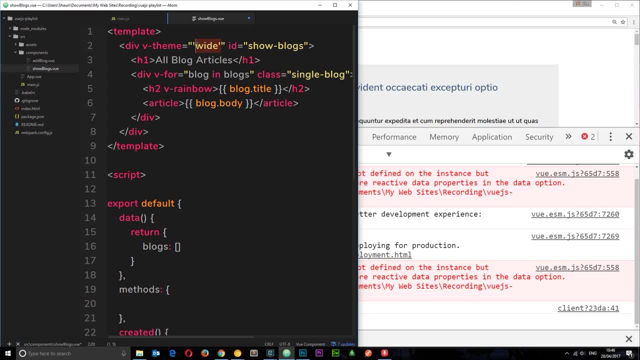 through in singles and I've got a string here, so I'm going to pass it through in singles and quotations. okay, this is a stream, because right now we can pass anything through here. we could pass an object, we could pass an array, we just want to pass. 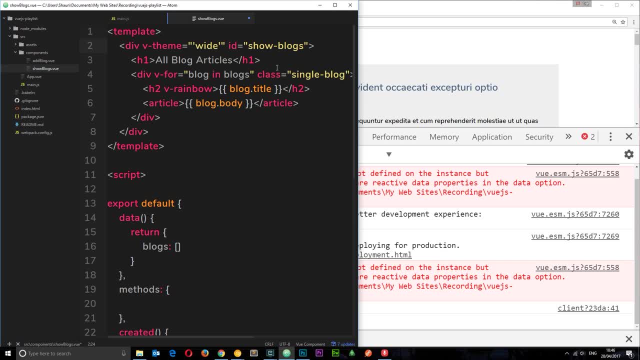 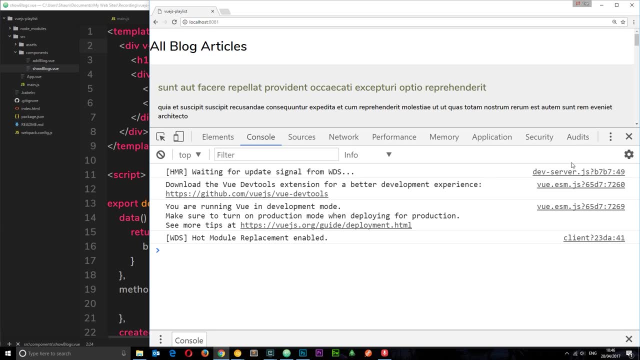 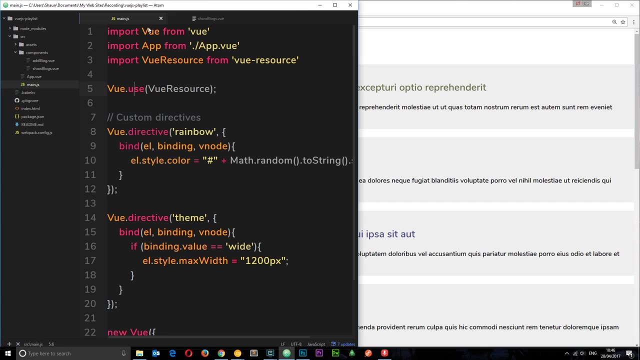 through a string. okay, so we're passing through a string which is wide, so let's save that now and see this works. refresh, and now we don't get any errors and we get the wide theme. cool. so what if we want this to be a narrow theme? well, we. 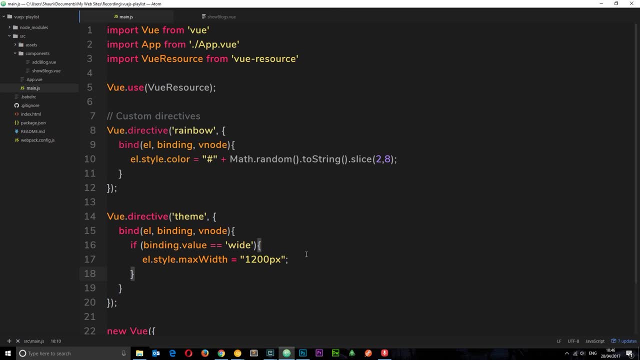 can do the same kind of thing. we can check to see if the binding value is narrow. so underneath this I'm going to come down and say else: if- and inside here we'll say binding- that value is equal to narrow, okay. and then inside here, if it is, we'll say L style dot max width is equal to, and it's going to be. 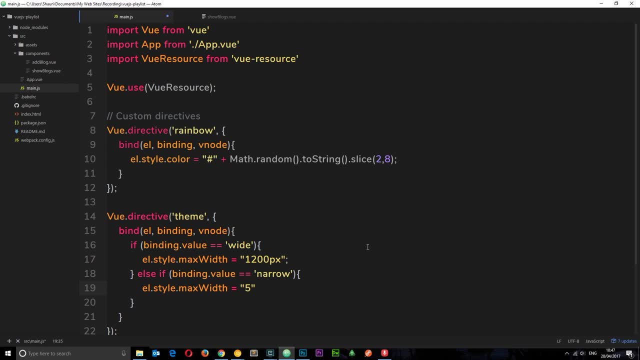 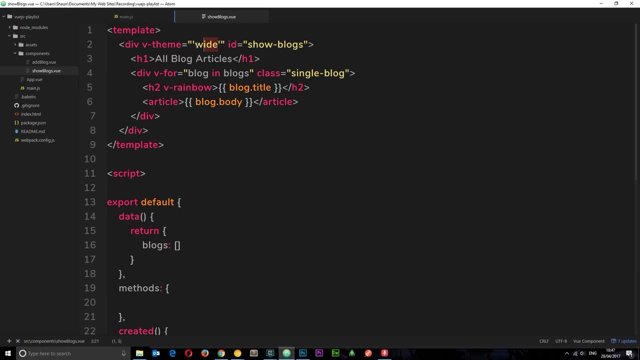 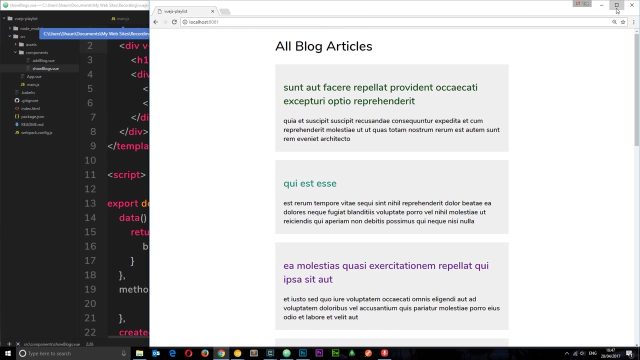 800 pixels, or rather something narrower. five hundred and sixty pixels. okay, so if we save this now and go to our show blogs and change this to narrow, save it. view this in a browser refresh. now we get a narrow theme. okay, pretty cool. so that's how we use values in these custom directives. I want to show you one more. 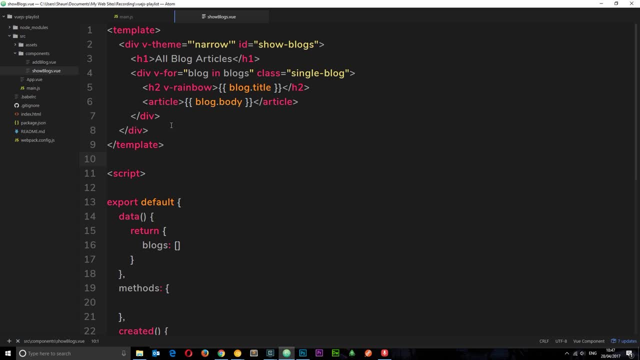 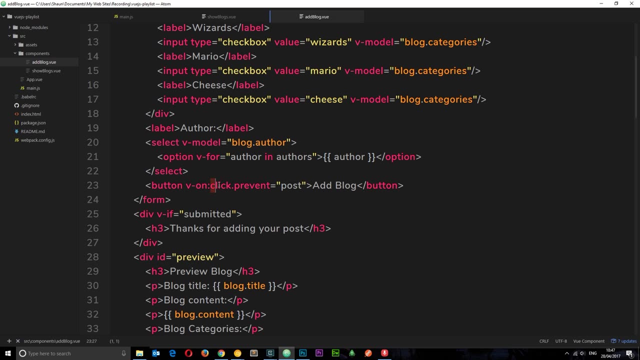 thing and that is arguments. so you know, like in other directives, for example, if we go to V on click this right here, colon, and then the click this is an argument, okay, so this is the value right here, when it's equal to something. and this thing after the argument- sorry, after the colon- is an. 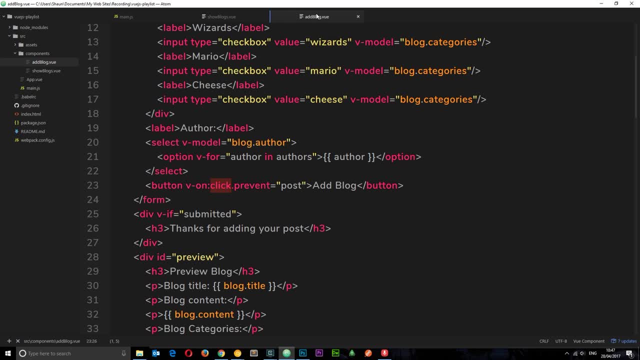 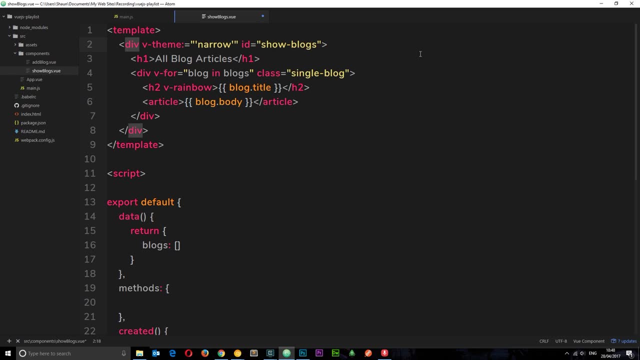 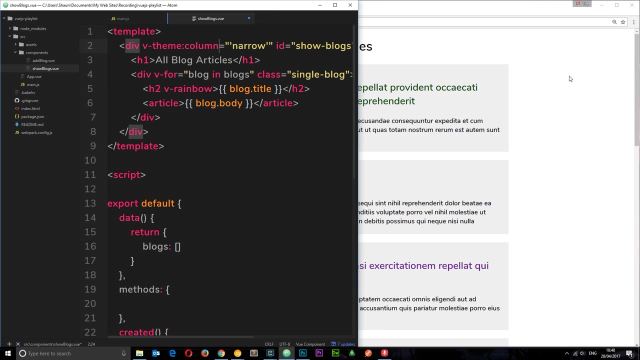 argument and we can pass in custom arguments into our custom directives. so say, for example, we want to pass in an argument to this, we could do a colon and then the argument name. so let's say, for example, I want to pass in an argument called column. okay, so we want it to look this thing like some kind of column on a. 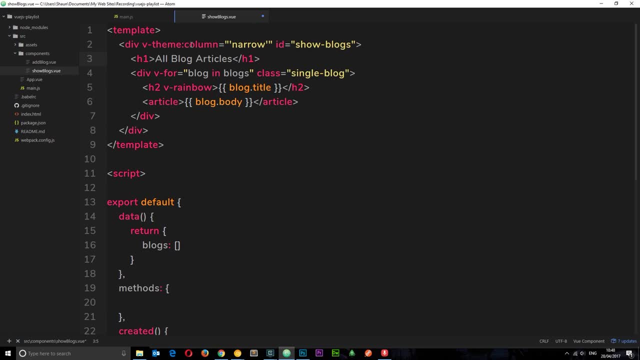 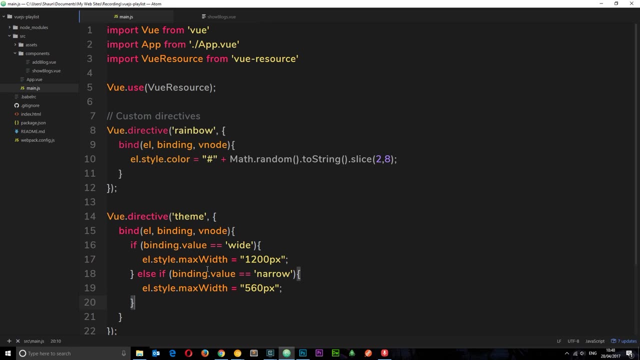 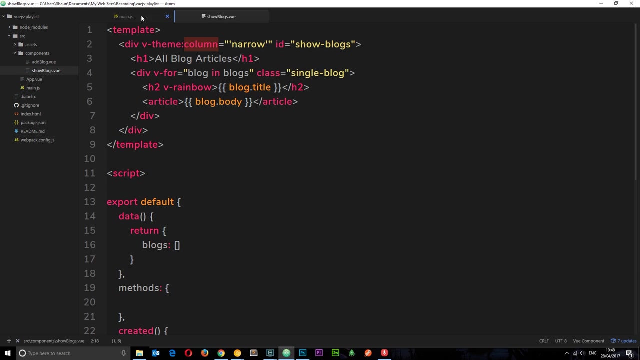 color, like a big strip going down, then what we can do is use this argument right here in the directive. okay, so what we'll do is also check. we'll say if, and inside the if statement we can check the argument so we can say if binding dot. 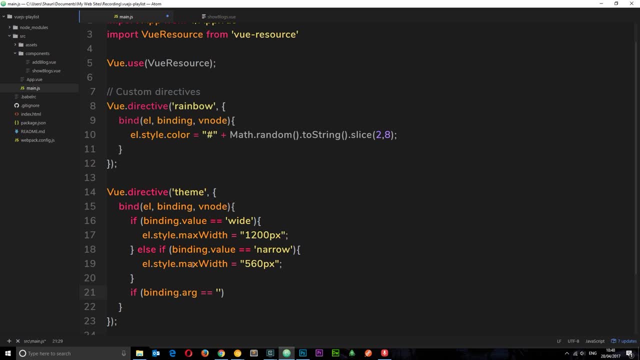 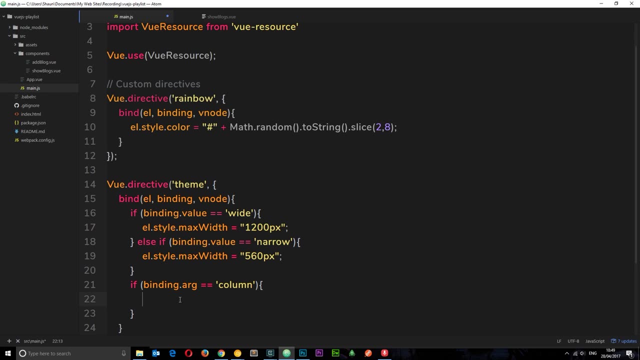 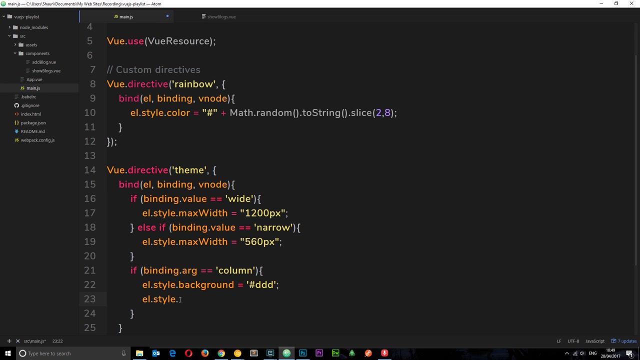 arg is equal to whatever we want it to be equal to, so column, for example- then we can do something much like we did in here. so we could say something like L dot style dot background is equal to- I don't know- DDD, which is like a gray color, and then also L dot style dot padding is: